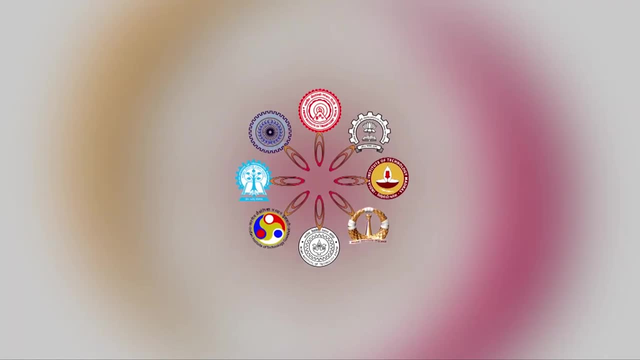 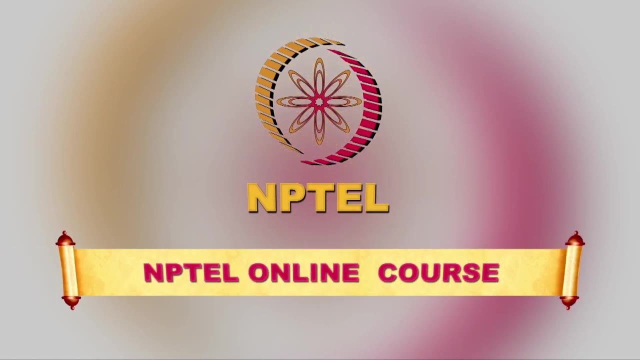 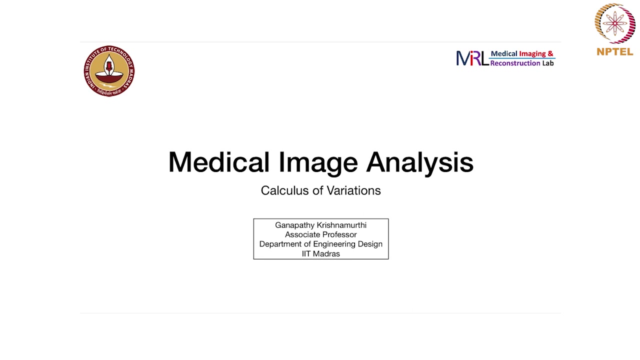 Hello and welcome back Today's class. we will talk about Calculus of Variations, which is a fundamental topic which is necessary to understand partial differential equations based techniques for image segmentation. So this is the calculus of variations is what gives rise to many of those techniques. We will have a brief look at this method just. 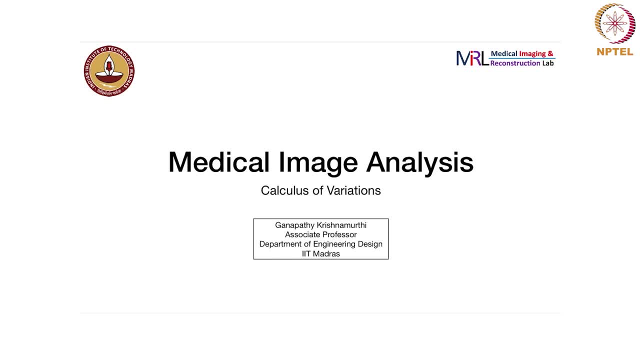 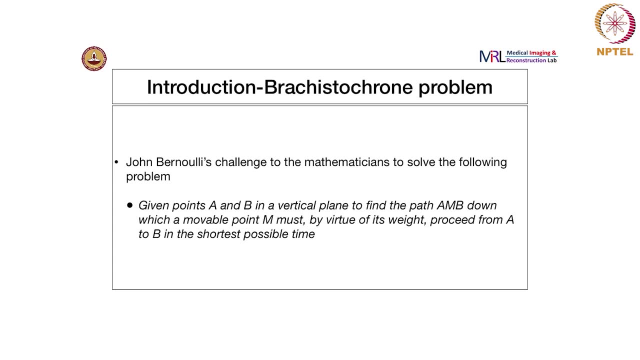 to understand where it comes from and the fundamental Euler Lagrangian equations. So we will look at the historical origin of the calculus of variations. So in the early 1600s, John Bernoulli, one of the mathematicians in Europe, renowned mathematician in Europe. 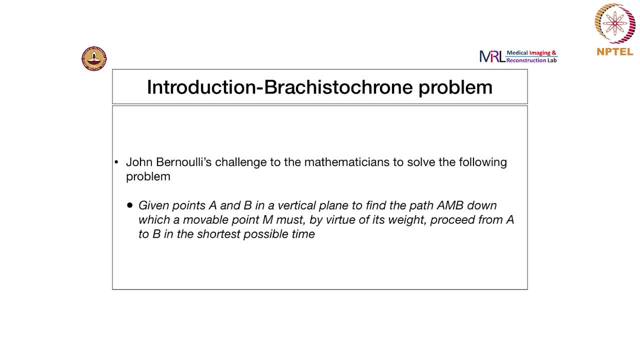 at that time posed the so-called Brackister-Crohn problem. So the problem statement is given below. I will just read that out. So, given points A and B in a vertical plane, to find the path A, M, B down which a movable point M must, by virtue of its weight, proceed from A to B in the shortest. 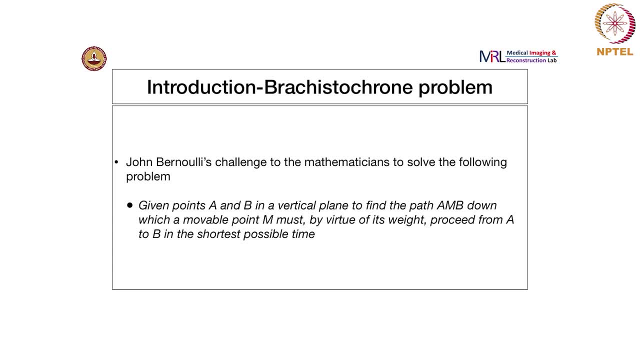 possible time. So basically it is a point- mass mass m, small m- and it is going to travel in the vertical plane. We will look at the images in the next slide From A to B. starting point is A, ending point is B and you have to find the. the idea is to find the path of that particle or B. 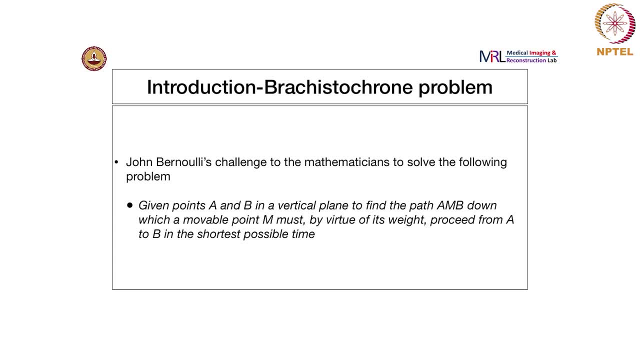 we take of it as a bead on a string. So find the path of that particle or a point, and it is. of course it is moving by virtue of its weight- means that the only external force is the gravitational force. right, it is acting downwards And the idea is to optimize for the time. 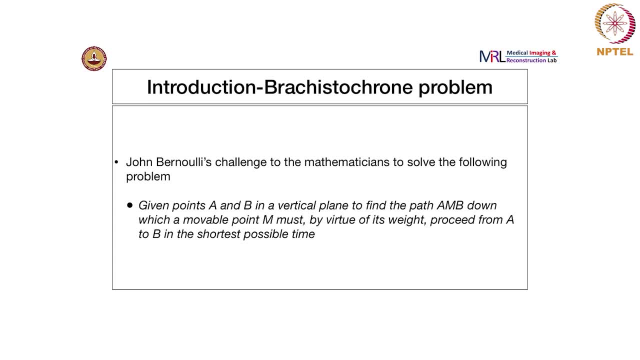 so you have to find out the shortest possible time, the path which gives you the shortest possible time, So that so this is like an optimization problem, except that the solution is not just one number or a coordinate, but rather an entire path or a curve, or a function right. 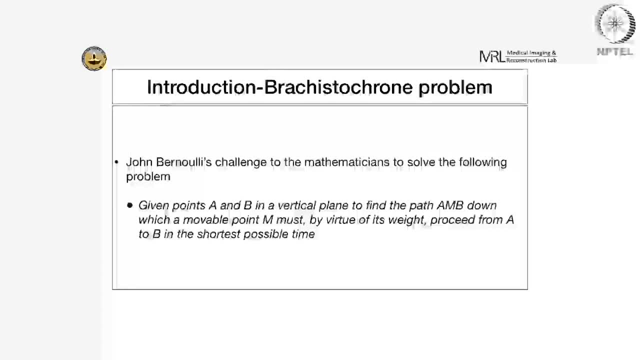 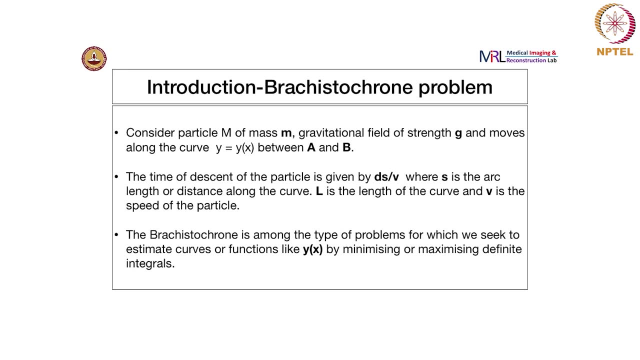 So we will deal. we will look at the details of this problem in the next few slides. So here is the slightly more detailed overview of the problem. So you consider the particle M of mass m. So the small m is the mass- your poor notation, sorry about that- But the gravitational 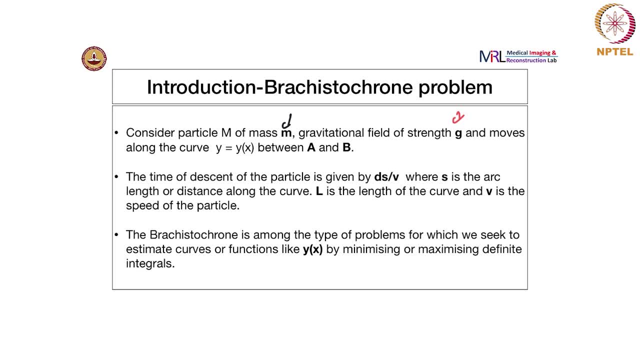 field of strength G. so this is the acceleration due to gravity right G, and it moves along the curve. the curve is parameterized by x, So y is a curve, y of x is the equation of the curve between two points, A and B, And of course it is in a vertical plane and the time of descent of 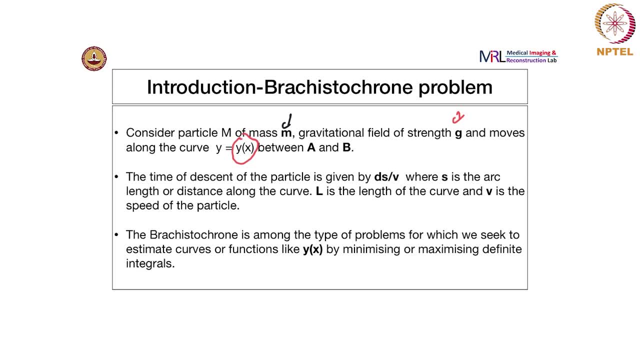 the particle is basically, if the particle travels along the curved path by an infinitesimal length- ds we call it the arc length, And the time it takes is given by ds over v, where v is the speed of the point mass of the particle, okay, And ds is the length along the curve. So 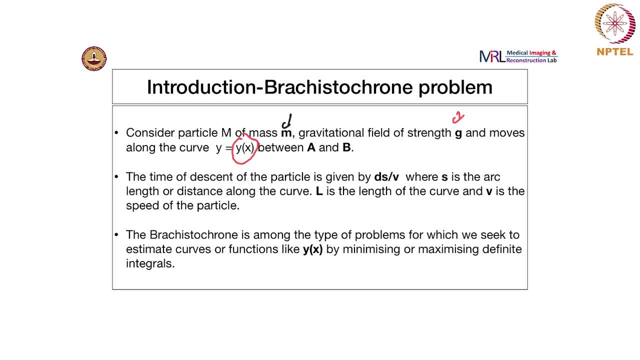 it takes a curved path, for, you know, general path is a curved path. So if it, if it travels a distance ds along that curved path, then the time taken by it would be ds over v, where v is its speed right, L is the length of the curve and v is the speed of the particle. And you can. 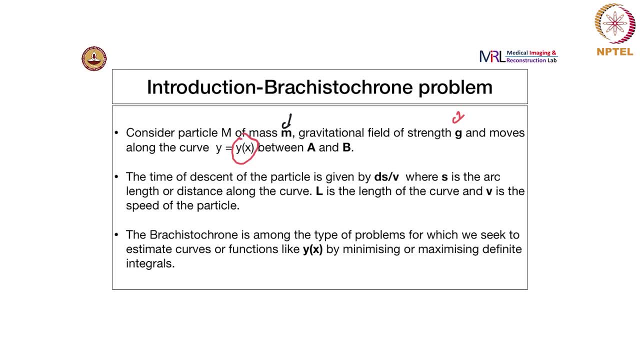 also denote the total time taken. if you think of it as T, right, that will be the total capital, T will be the total time taken. So this is the problem statement. So we are trying to optimize for time, So we have to find the path that gives the shortest time. So, if you have looked at 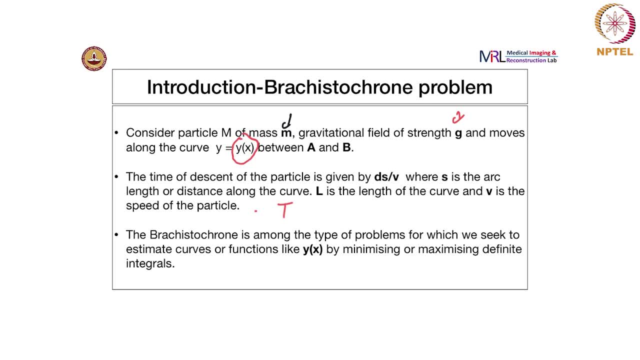 optimization problems before. for instance, you know, in neural networks we are looking for parameters that provide the smallest loss function right. In a lot of cases in optimization we have some form of cost function and usually try to estimate parameters in that optimization problem so that you know the cost. 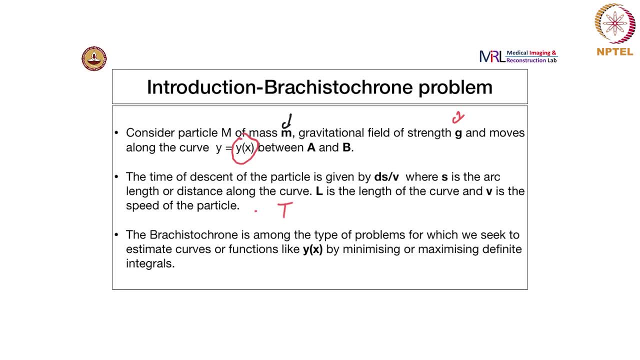 function or loss function, is small Here. the loss function, if you want to think of it, is the time taken. Time taken should be just as minimum as it can get. And what parameter are we trying to estimate here? We are not trying to determine a parameter. rather, we are trying to determine an. 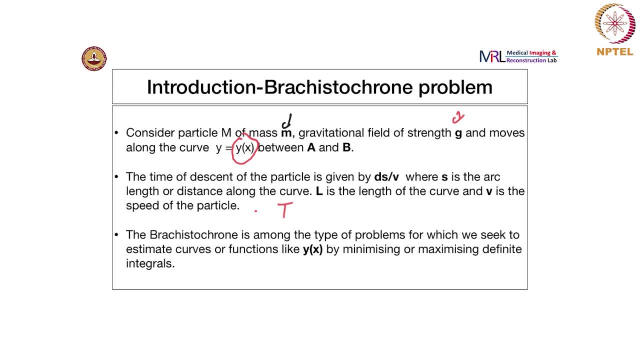 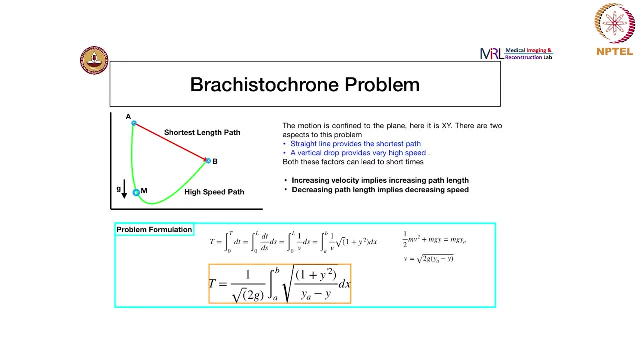 entire curve or a function. So these are the kind of problems you know that is concerned in the field that you are concerned with, in the field of calculus, of variations. okay, So we will get slightly more. you know detailed, look, because I haven't shown you any. 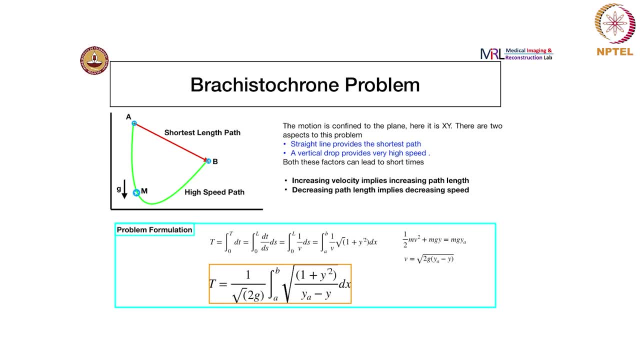 picture. so far, just talking about these things. Okay, so, without any loss of generality, we can say, okay, and this is, this is the vertical plane, right, and think of this as the y axis and this is maybe X. so and you are, you're trying to get from A to B, right? 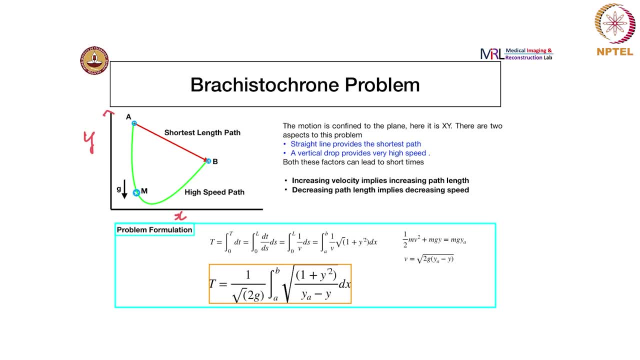 in the shortest possible time. so what is the path? what is the curve that will take you from path, or curve that will take you from A to B? and this M here. this is up. this is the point mass you're talking about. G is the acceleration due. 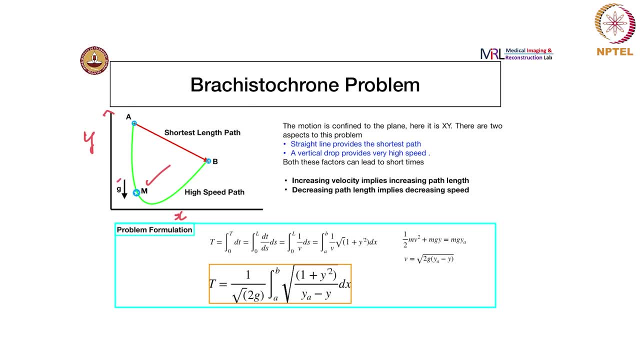 to gravity. so, um, so we are trying to estimate this equation of this part, right, and you call this y of X. now, how are we, how do you go about doing this? so if you do cut it intuitively, then you know, you would immediately say: let's. 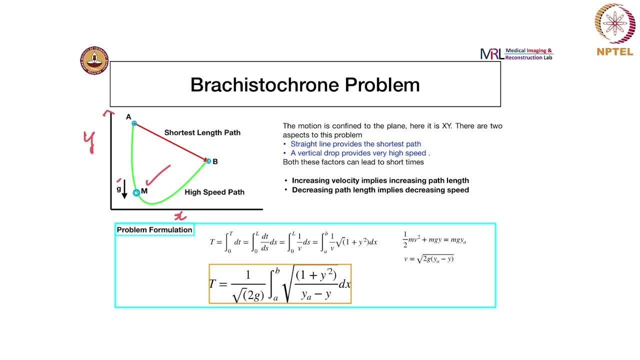 choose the shortest path. the shortest path is the straight line between A and B. that's what is given here. this is the straight line. so if you look at it, this is the straight line right. so ideally you would think of the shortest path- straight line path would give you the least time. but also think of it the other way. if you let the 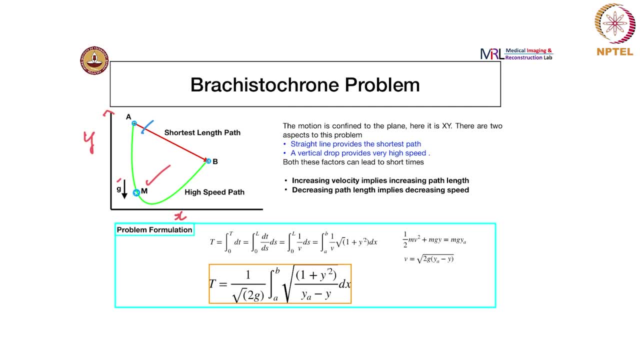 particle. drop a bit vertically, quite a bit, then it will gain speed. right, whether it's motion under gravity, it will gain speed. so you're not giving it any extra moment, I was just dropping it, so it will gain speed. and so then, if you think about it, in which case the time is still can be reduced because you have higher. 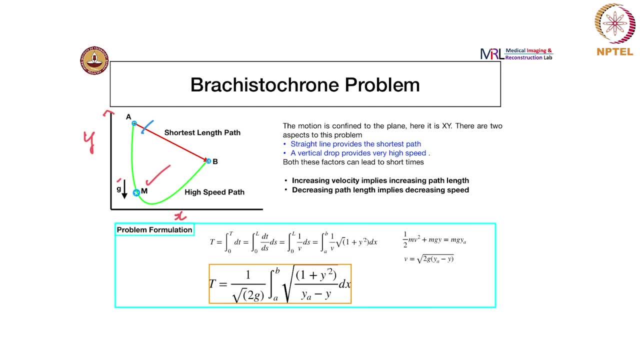 speed. but the problem with this approach it is that you let it drop a bit vertically downώραアfö. you know we have a longer path right. so if you want to increase the speed or velocity, it is get nervous slightly longer part, but it will be very high-speed so that 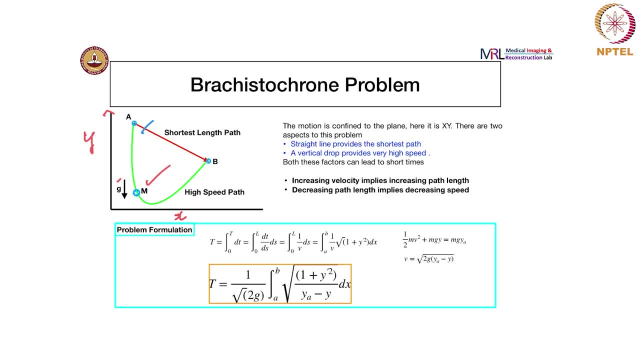 you have a good chance of getting reaching that quickly from A to B quickly. on the other hand, if you are just choosing the shortest length, then maybe velocity is not that great and typically is like that right, and so then you might not get there. and even the one, though the time-out is relatively graceful. 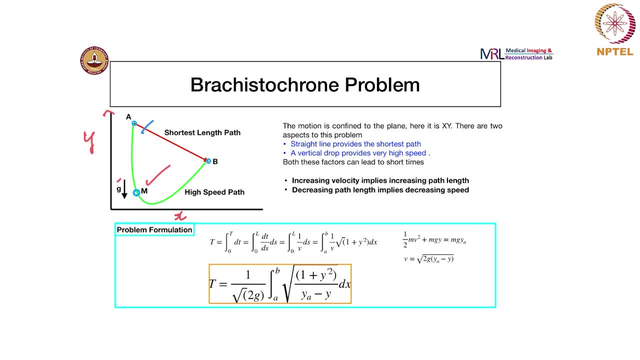 might be reduced because the path is shorter, but they are still not very clear. So there are two things at tension here: Longer path, high speed, shorter path, low speed. So we do not know which is better. Now you have to find a compromise between these two, So many of the problems we 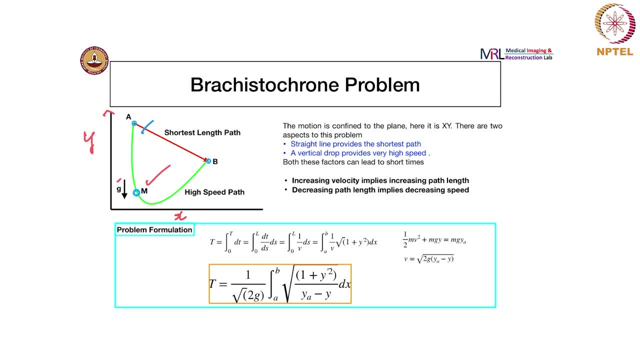 will talk about segmentation problems. we will talk about this kind of tension will be there between two different quantities that we are trying to minimize, right, So that is, and those situations is where, you know, calculus of variation comes in handy, So it provides you a 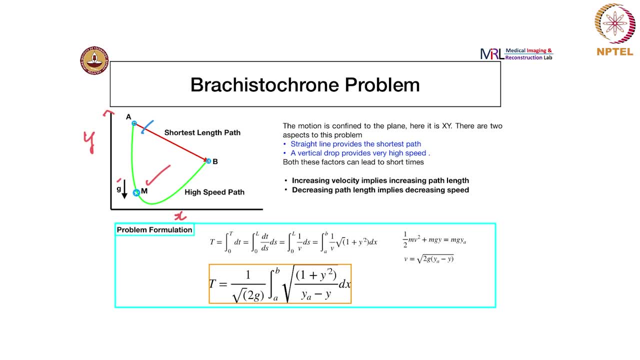 systematic way to arrive at correct solutions. okay, So in this case, what we are trying to figure out is the equation of this curve. So, mathematically, the problem is formulated as follows: So we want to minimize the total time taken, which is what this integral gives you. 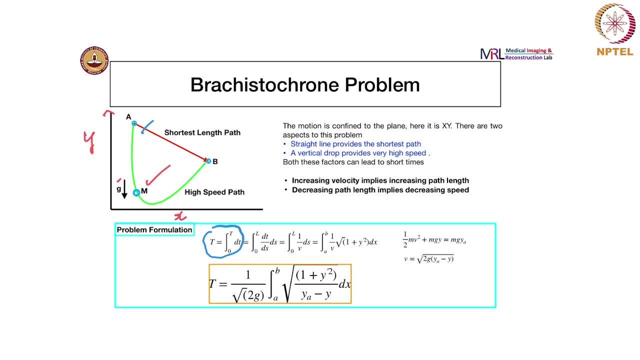 right And we saw that dt can be written as ds over v and that in turn can be written as 1 over v, square root of 1 plus y prime square. So what is y prime? Y prime is nothing, but y prime is dy by dx. I will. 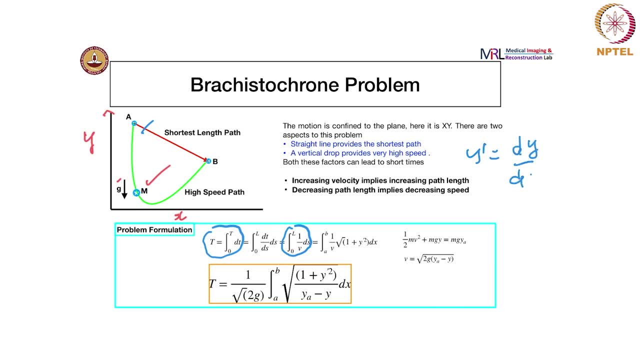 just write it out here: This is a very common derivation. You can actually google this and you will find it everywhere- Wikipedia pages for it. So I am not going to go into detail, but eventually you have to do a few substitutions. 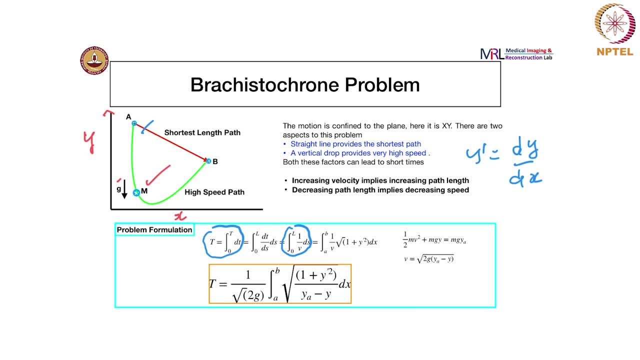 Basically for the velocity also because the v you can get by conservation of energy, right? So if y a is the, maybe I will have to zoom in a bit. So y a is the position of the starting point. 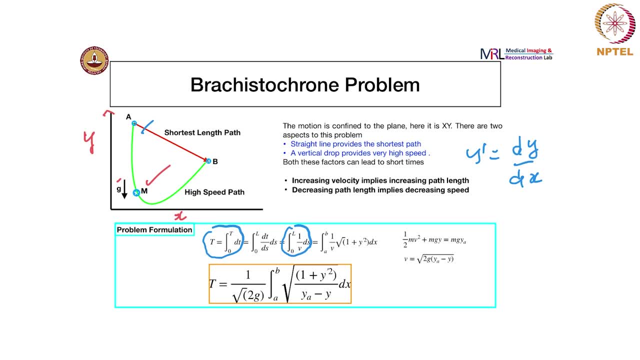 right. So this is the starting, the coordinate of the starting point, y, a. If it drops a distance, y, then it gains some kinetic energy. okay, So your initial energy is purely potential. So, using this equation of energy, you can evaluate an expression for v from this equation above, right. 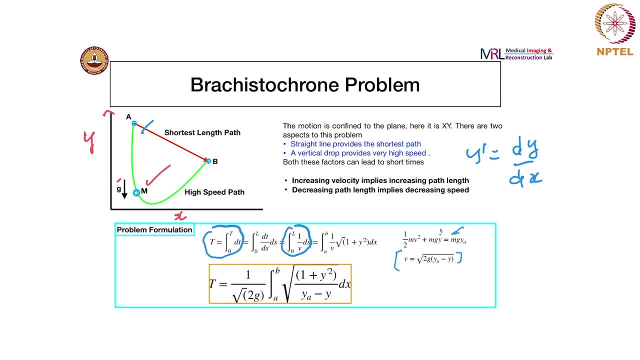 and then substitute back in the integral, So that will give you this integral expression, an integral expression for the time, a definite integral expression for the time which is 1 over square root, 2g, and integral a to b and whatever is in this practice. Of course, this on the numerator. 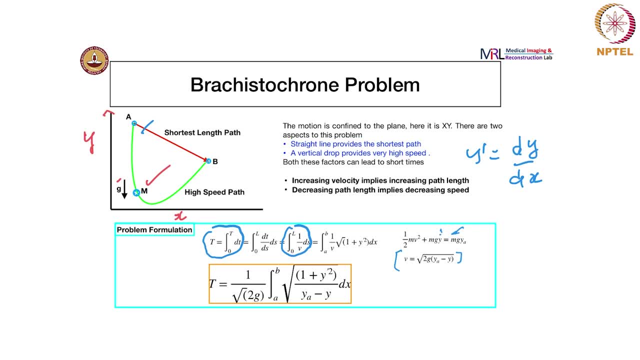 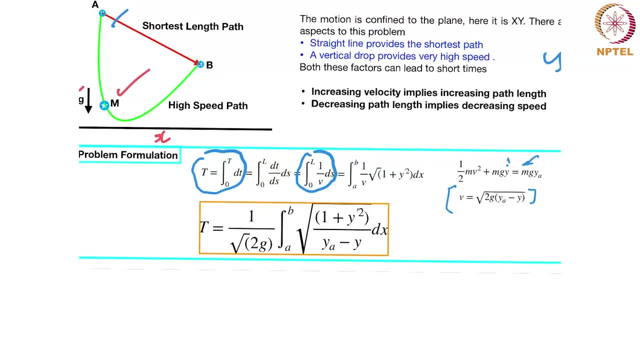 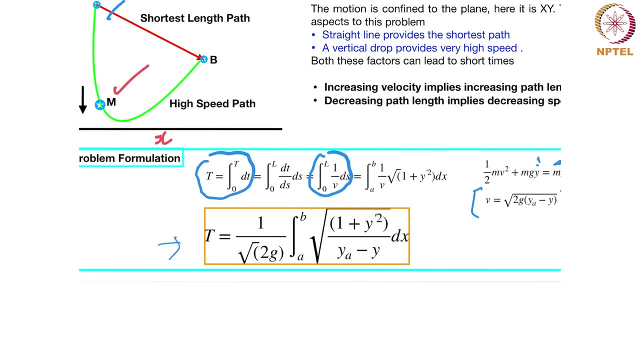 this is y prime square. okay, Just keep that in mind. Maybe I will zoom in a little bit just to make sure that. So this is the integral that we want to optimize, right? So you want to find the minimum time. 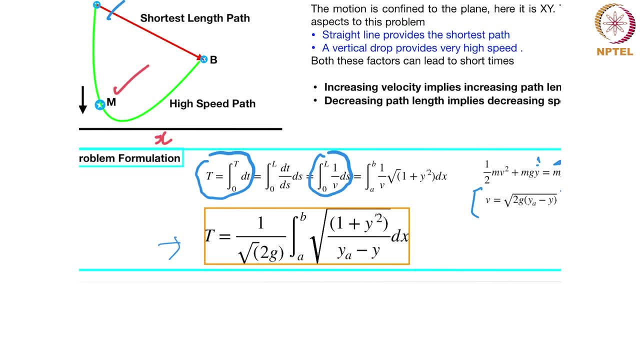 okay, So this integral is what is referred to as the functional. So this is the functional. So functional takes as input a function, in this case a curve, and returns a scalar value. So in this case it is the total time taken, and we want to minimize the functional. 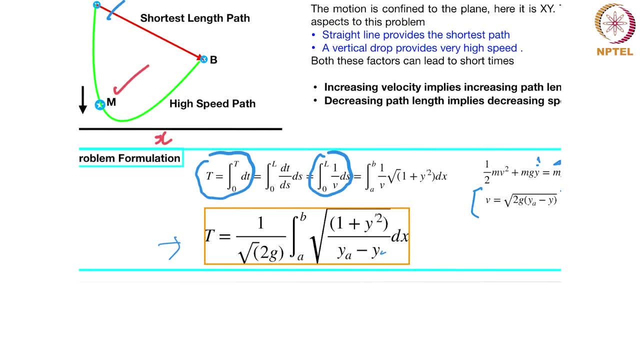 To arrive at an optimum path, which is basically y. we want to figure out y of x. that is what we need, So we will. we will revisit this once we finish derivation. okay, If you want to minimize time, which is basically: this is the functional. 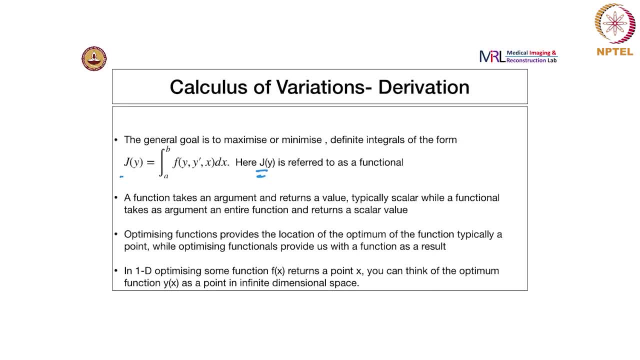 then you have to find a path y, So it is entire function. So okay, so the the general goal here is to maximize or minimize definite integrals of this wave. So you want to do- and I am not grabbing you, I am simplifying it- You are navigating between the cycles here. What you need to notice is to get. the m equal to 0, okay, So you need to draw some graphs, So the約 gallons which are out, And you have come and you have just played with the definite integral of that function and to get in that點 in. 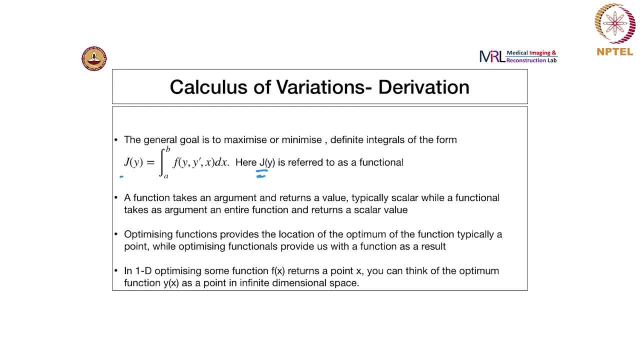 integrals of this form. So, if you note, it is a definite integral a to b and f here, with the integrand is a function of y, y prime, which is dy by dx and x. This j of y itself is referred to as a functional. So, like I had said it earlier, a function takes an argument. 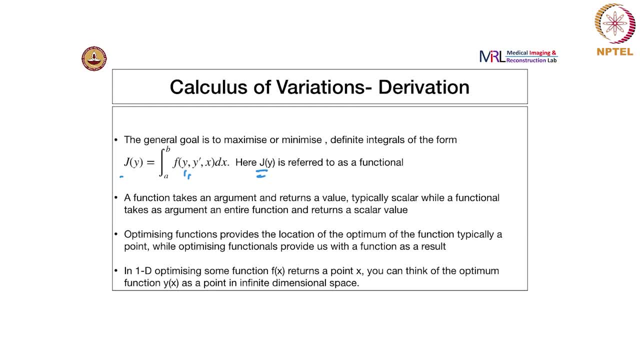 for instance, if it is a 1D function defined on a real line, let us say, takes as x an input on the real line and returns a value which is typically under scalar on the real line- Typically a scalar- while a functional, in this case, takes as input a function, the input to 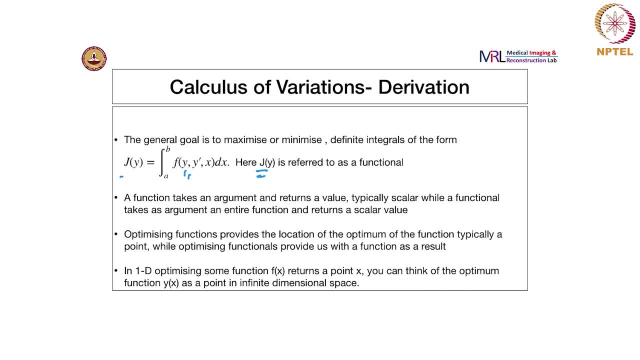 this functional is y. y is a function, it is a curve, but it is still a function and returns a scalar value. So when you optimize functions, what it does, it provides the location of the optimum. So let us say f of x is x square. let us say you are optimizing something like: 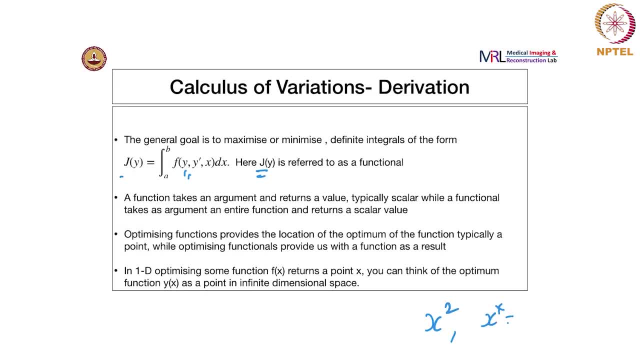 x square. The location of the optimum is x star equal to 0.. That is where the function f of x takes its lowest value. So in this case, when you optimize this function, what you are trying to do is to estimate y, the function itself. So you 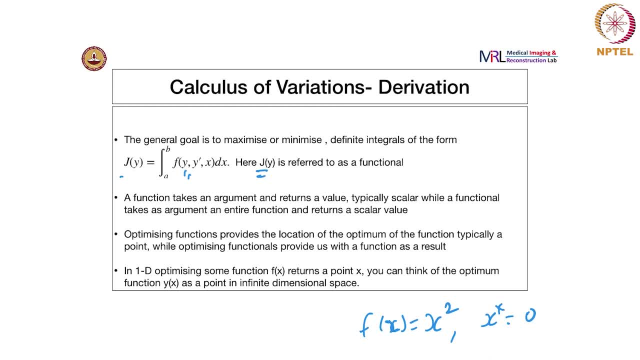 want to estimate a function which will optimize this function. Now there are some other aspects. like you know, this is actually defined in, you know, infinite dimensional space. because if you look at this typical function optimization, let us say 1D f of x equal to x square. now 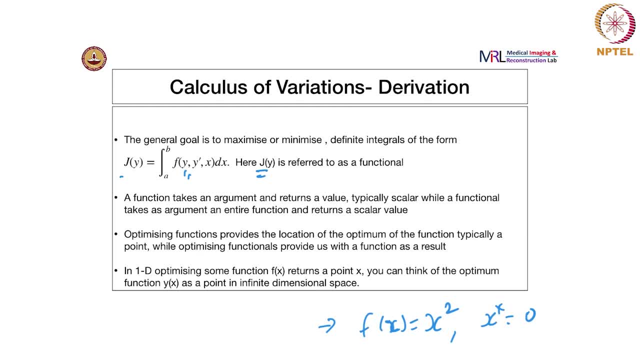 x is just in one dimension. But when you consider trying to estimate an entire function, then the problem is defined in infinite dimensional space. here again, infinite dimensionality comes from how you represent the function, what basis you represent the function. So, for instance, if you use a Fourier basis, or you are using Fourier series or Fourier transform there, 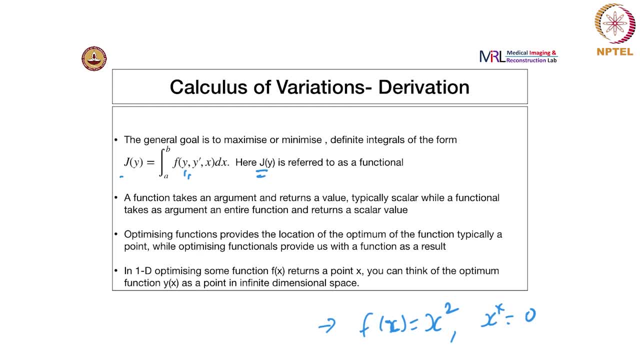 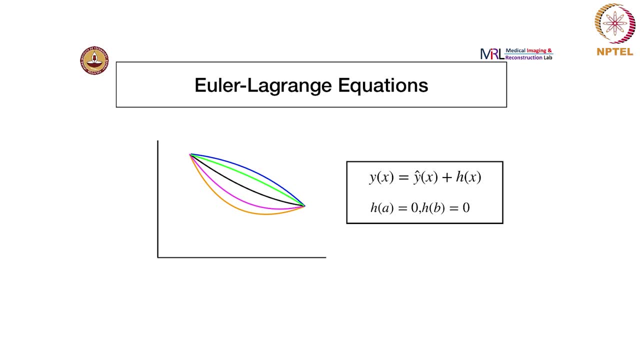 are infinite number of terms. So, consequently, you are in an infinite dimensional space, making the problem lot harder, Okay, So just to reiterate, so let us consider this picture here and I will try to tell you what we are trying to explain here. So let us assume that you know the solution to the 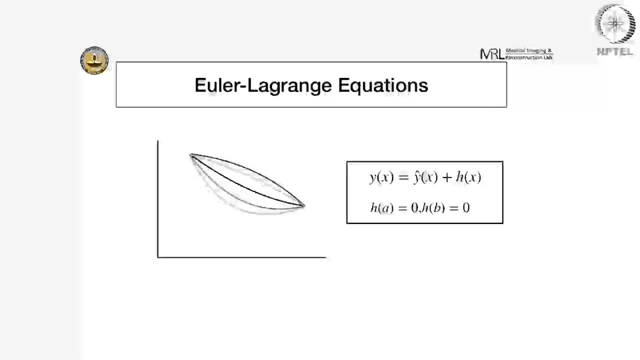 problem we studied right. So let us solution here. let us just: this is x and this is y solution we wanted So the solution curve, which is basically the curve that we want to estimate from a to b. So I put a here and b there. okay, So b is: 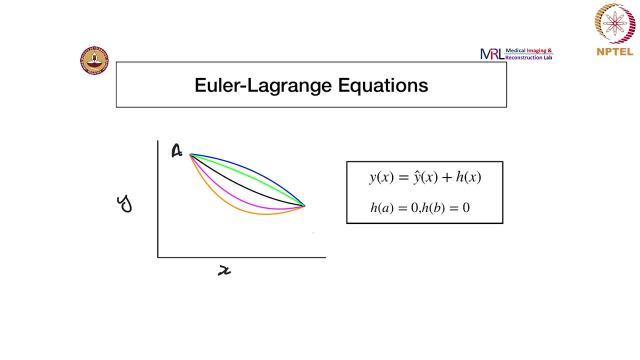 slightly around that of so b, So b here. and let us say the black curve is the correct solution, right with the curve that gives you the shortest time of travel from a to b. So that is the black curve. I have to use some color that I have not used here, So I just 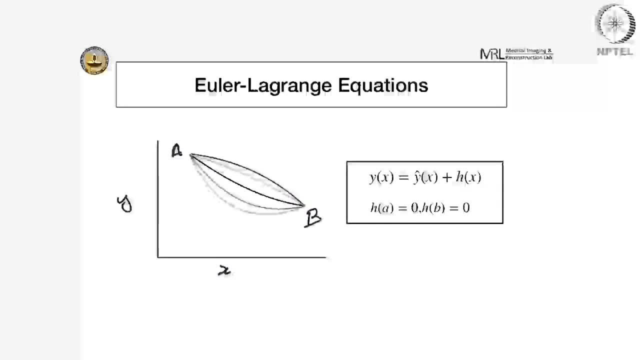 stick to the black here. So black curve is the correct solution, right, that is the one right here. that is correct, okay, So we all know that. see, when you, when you work with minimization of functions, etc. Let us say we have some we are now talking about. 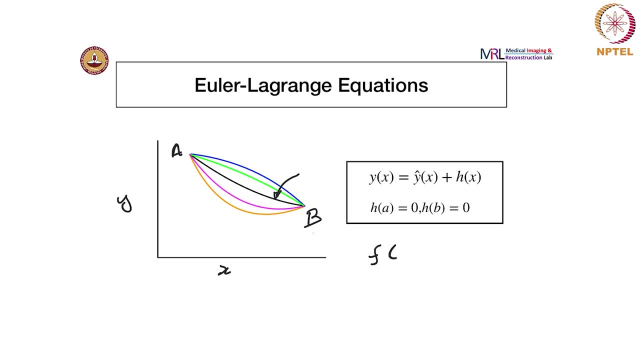 a different topic. So let us say we have this function f of x, right, And this is defined on the real line. So x is probably minus infinity to infinity- take on all values on the real line- and f of x is scalar valued function. output is also a scalar, okay, So 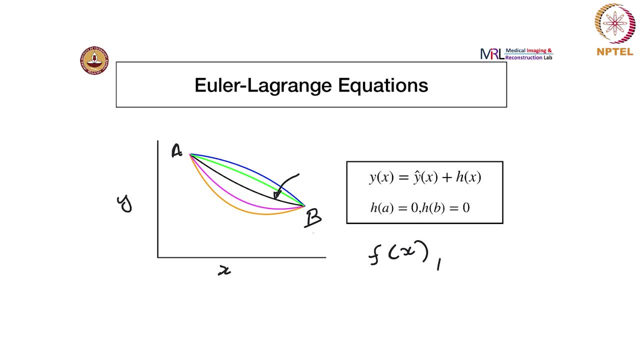 it returns a scalar. So let us say: x star is the point at which f of x attains a minimum. I will just talk about minimum, right? So x star is the x star is the x at which f of x becomes minimum. So if you look at any perturbation around, 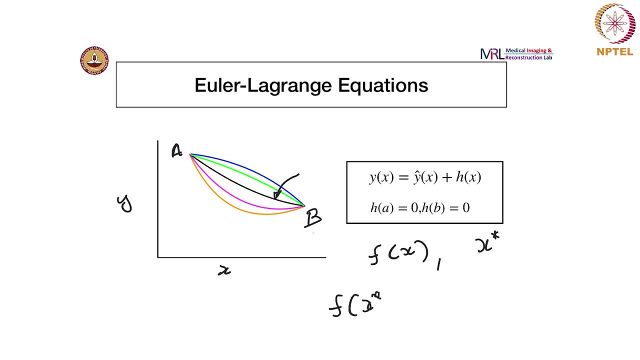 x star. So if you look at, let us say, x star minus delta x, and also you can do f star, f of x star plus delta x, small perturbations. maybe you have to rewrite x star, f of x, So f of x is a bit. So if you look at this then you see that for all these values, when you 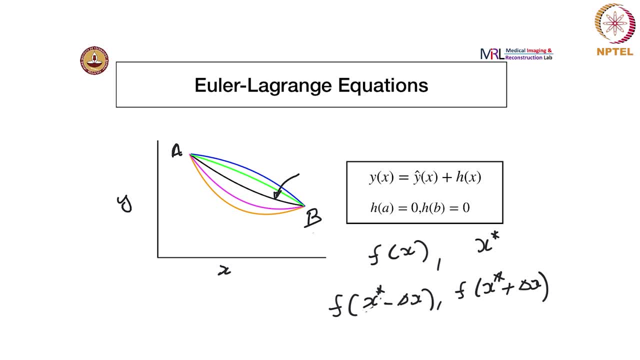 move to the left a bit or to the right a bit, since x star is the minimum. But there are other assumptions here. I am assuming that there is only one minimum for f of x, right global minima and no local minima, etc. We have to make all the necessary assumptions. 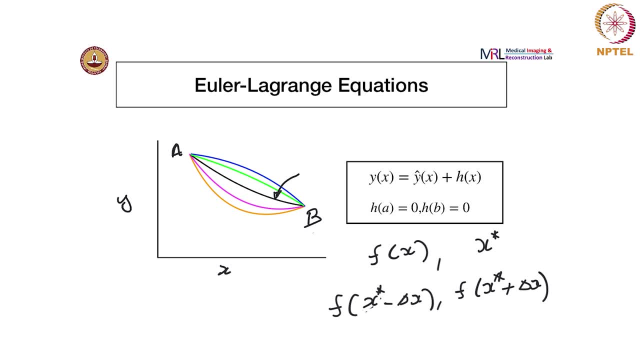 right, But then still we are only looking at the neighborhood. So x star minus delta x and x star plus delta x, if you move either to the left or the right, then f of x in that case for all. if you f of x star minus delta x and as well as f of 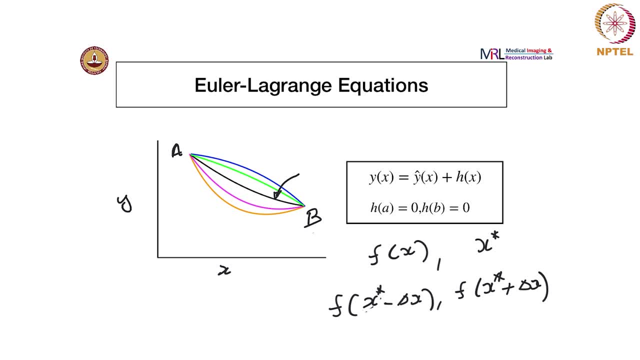 x star plus delta x and everything in between except for x star, will be greater than the value at f of x star. So all value of f of x In this case what will happen is that escape on x star will be greater than or equal to. 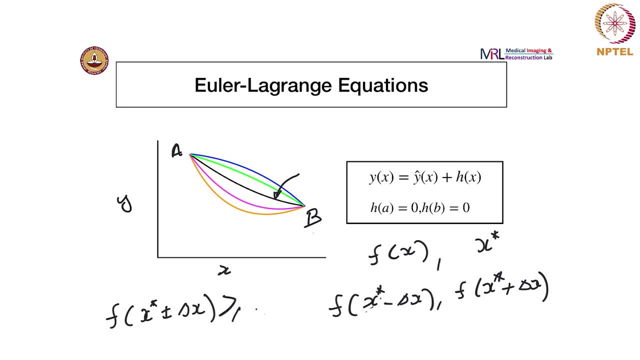 f of x star, right. So this is true, right. If your x star is the minimum, gives you the minimum value of f of x and it is that x star and then if you perturb it, perturb the value of x around x star. 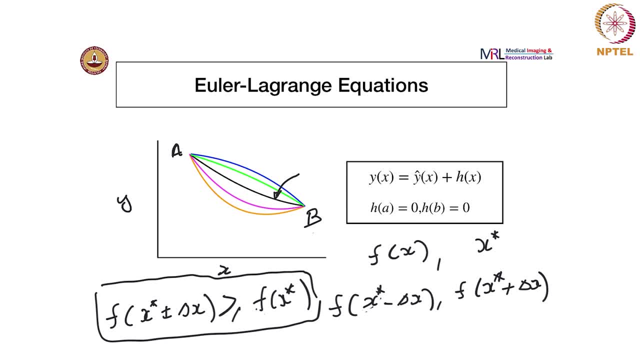 Then all values will be equal to f of x star. And now the ந and Además n掰 is known Right. So now this is not true right, because x in x is the minimum limit now you can do all. f of x will be higher than that. right will be greater than that. So it is very simple. if you 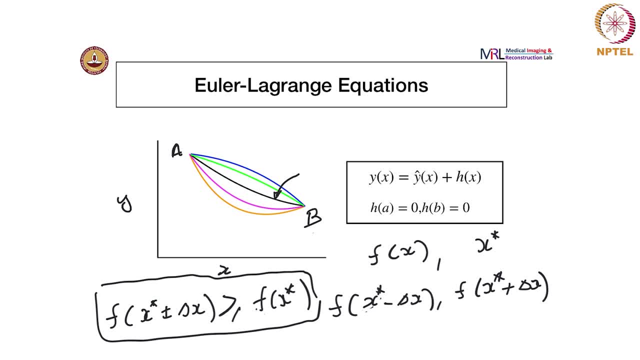 let us say, if you draw, let me wipe this out and draw so it is easier. Very simple function like this parabolic function, right. So if you are, if this is your minimum, right there, if you move to the right or to the left. 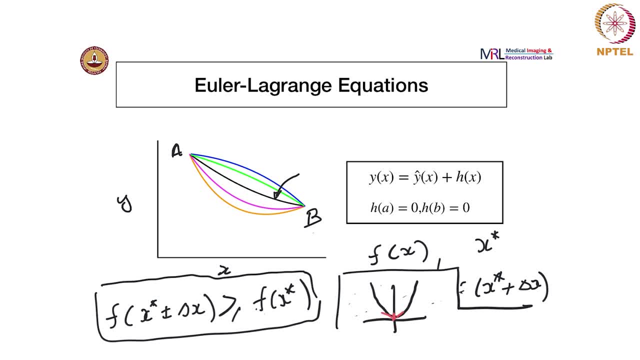 the function value increases. that is what I am trying to say. okay, So similarly, but then this is in, you know, in the real axis. of course you can also consider it in multiple dimensions: x, y, z or x1, x2 up to xn, but the argument remains the same. if you perturb it a little bit, 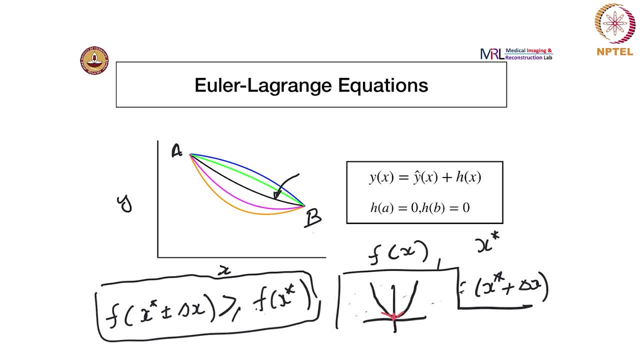 around where it attains its optimum value, in this case its minimum value, the x values, the coordinate values, then the function value will increase, right? So how do you do similar things? So how do you do similar things? So how do you do similar things? So how do you do similar? 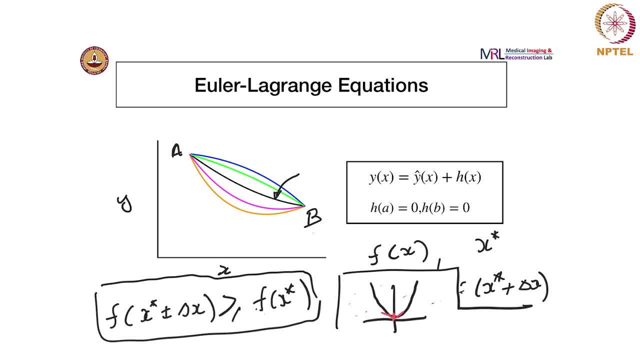 perturbations in. you know when you are trying to estimate function. So if this is our correct optimal function, right, if this black curve is our y hat of x, this is the path that gives you the shortest time in our problem we are studying, But in general, for any such definite integral, we 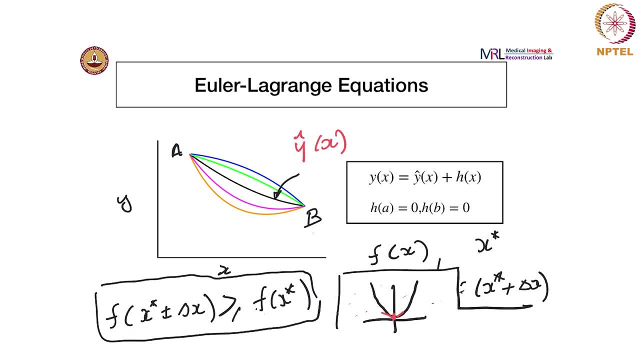 saw. let us say, this is the function that gives you the least value of the functional, then how do you perturb this? So you perturb this by adding a test function: h of x. right, that is how you do Here. you added delta x, you are adding h of x, And it should. 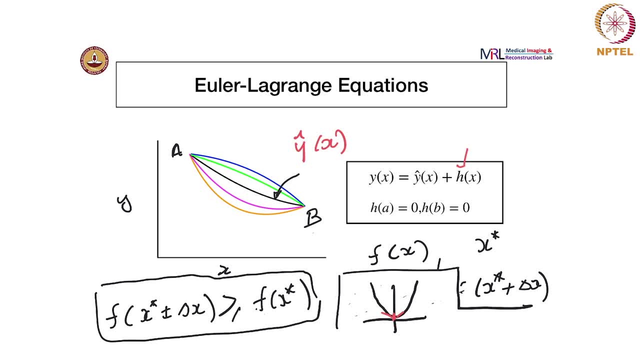 of course, satisfy the boundary conditions here, because boundary conditions is that you know it is. in our case the particle or the point mass starts at a and ends up at b. okay, So the boundary condition it should satisfy, so, which means the h of a equal to 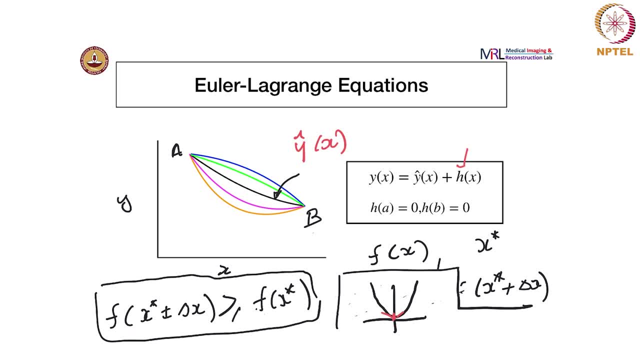 h of b equal to 0, so that at the ends of the path you know your boundary conditions are met. And this is true for any other problem. there will always be a boundary condition and you have to meet them. this is one way to meet it. So h of x is a think of. 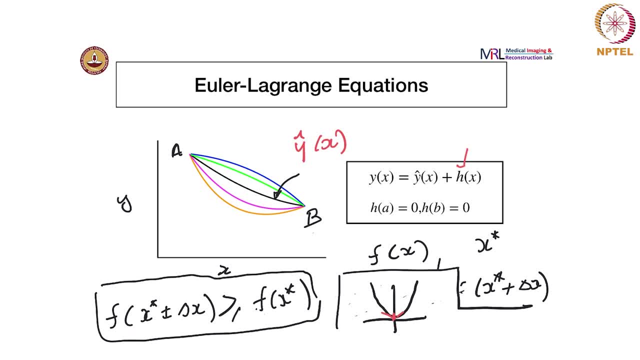 h of x as a small perturbation to y hat of x, which is the correct or the correct curve that we are seeking. okay, This is how we perturb it, right, because it is like you said it has. 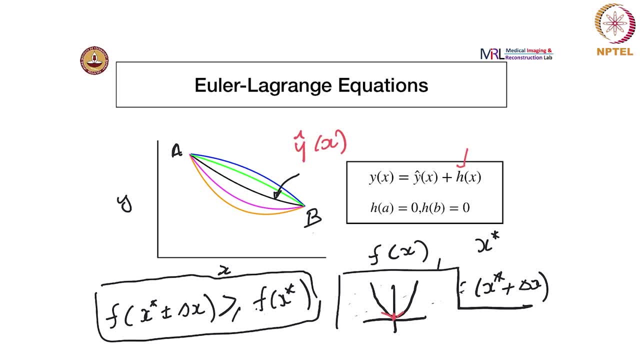 it is an infinite basis or infinite dimensional space. So only way you can perturb y of x is by adding another test function to it, right? So this is, of course, this is the important point that you have to understand in the calculus of variations: that how do you perturb this. 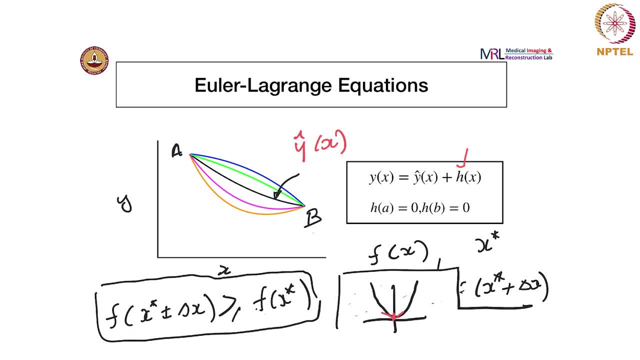 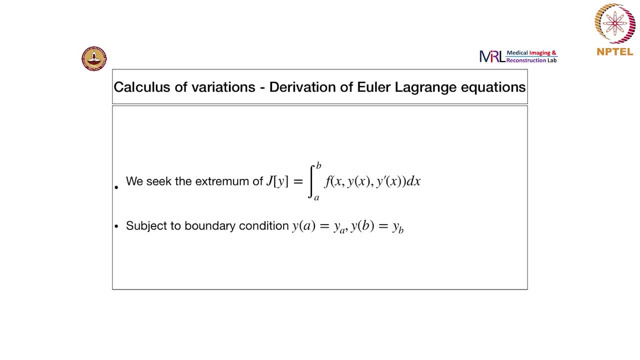 function right, And we are not done yet. So we will have to look at you know what we will. further calculations are required in order to arrive at the so-called Euler Lagrange equation. okay, So we seek the- I call it the extremum of j, of y. So we just you know, but you have to pass. 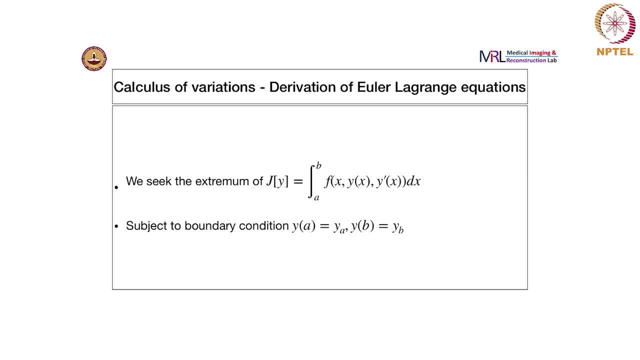 this in your mind, saying: we seek to find some y such that j of y attains a minimum value, okay. Or you can also say maximum value, but you can always change the sign into that: okay, And there are boundary conditions to be met, such that y of a equal to y, a y subscript a and y of b equal to. 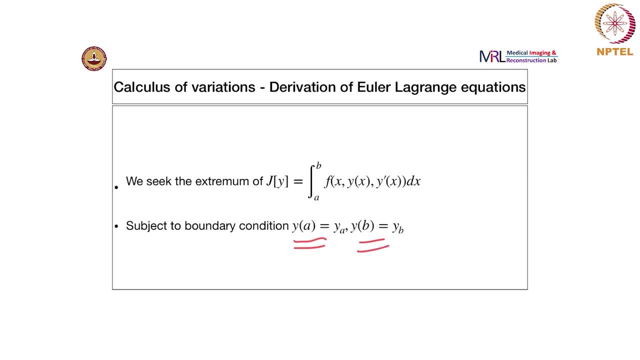 So you understand that. And the integrand is some function which is a function of x, y of x and y prime of x. Sometimes you can also have higher derivatives, So y double prime of x. We will see that This actually happens in some of the image processing problems. So we will see it. 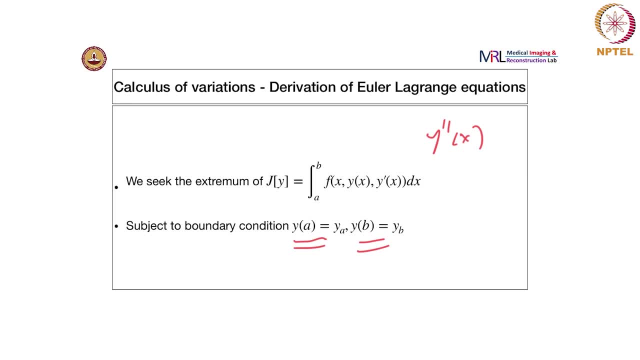 we will see about that when we get there. okay, So we seek the extremum of j, of y, That is what I call it, extremum. Once again, you know this optimization literature has, you know, different definitions et cetera. So I am just being very informal. So, 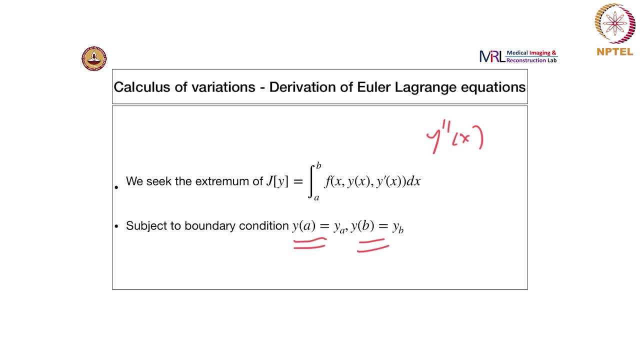 so do not hold me to this, okay. So I assume that we are just trying to find out y, such that j of y is minimum. This functional is minimum. right, That is it. So, like we said, we have to. 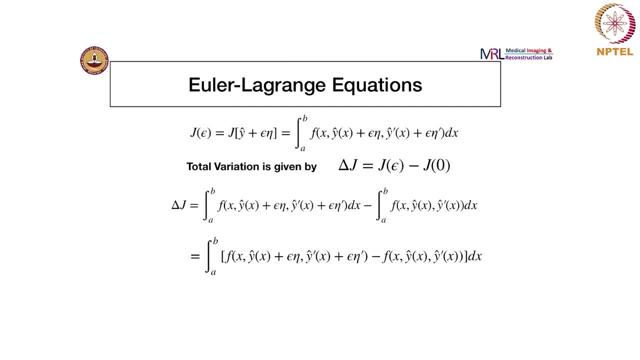 perturb it around the optimal solution, right So? which is basically: we assume that y hat is that function for which j of y attains minimum value. So we then try to perturb it. That is what we do, right? This is again a familiar trick, You remember, when you also try to take derivatives. 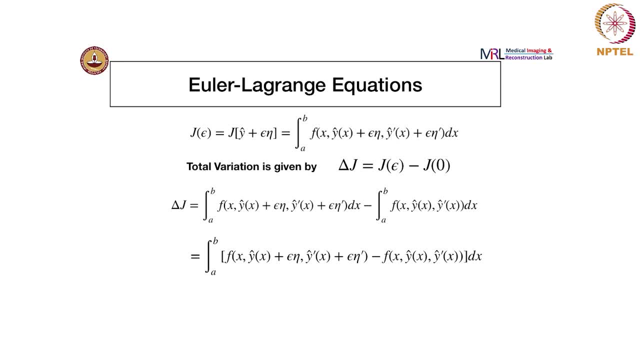 then we do something like that, right? So we have an infinitesimal change in the arguments and then we try to see how the function changes, right. Similarly, that is what we are trying to do here, except that we have to be, we have to parameterize carefully. So we saw that. 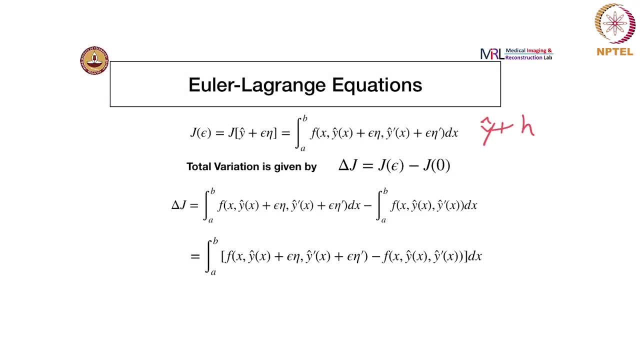 you know we are trying to. in the previous slide we tried to do y hat plus h, right. That is much harder to do, actually right, Because what do we eventually want? We want to ever have estimate this right. We want to estimate right. So that is what you. 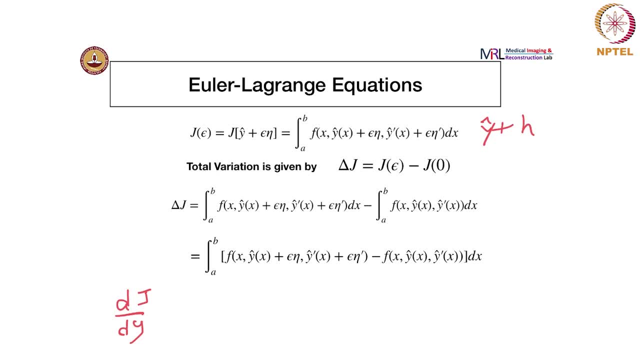 would do If you want to find out the maxima or minima of, let us say, arbitrary function. I am using f here all the way, but you feel to put something g or you know if you want h also. So if you would do differentiately to d, f by dx and set it to 0, this will give you a. 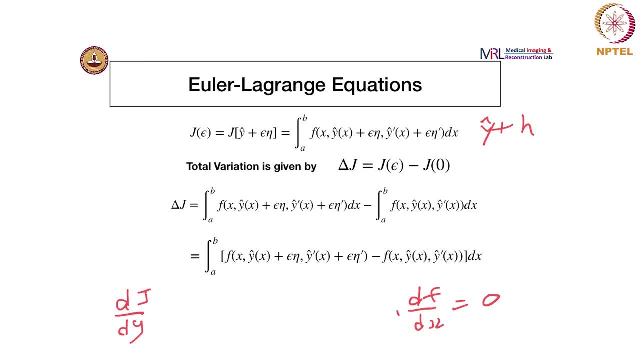 maxima or minima and you will look at the sin of the second derivative, like, and you will also examine the sin of d square f by dx squared and that will give you whether it is a maxima or minimum. But in either case, this is the first step. You have to set the first step. 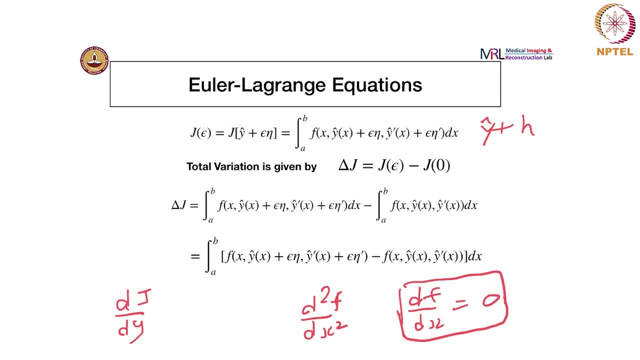 this to 0, right, And the way you would do that. now, if you want to thought on principles, then you will perturb f of x. you can write as f of x plus delta x, etc. So we want to write dj by dy. 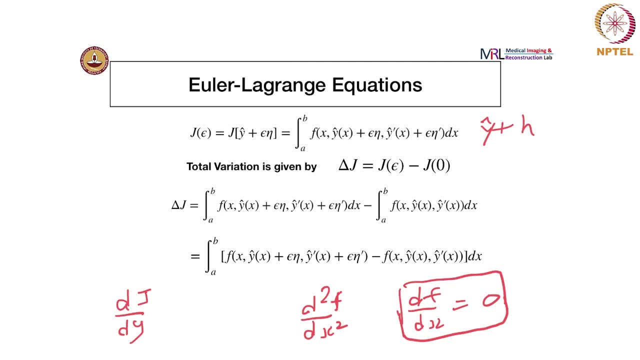 and this is hard to compute using just this. you know this kind of trick right. But then we have to perturb everything by h, and then h prime, and then we have to say h, h is small. So because when you do f right, this kind of derivative you will do by f of x plus delta, x minus f of x. 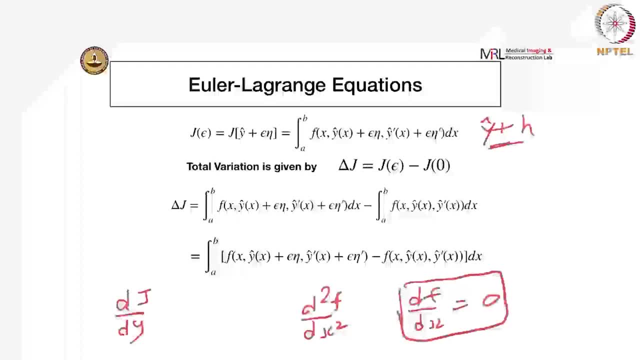 right, something of this sort. I do not want to write too much around here. just to give you an idea. So you will do f of x plus delta x minus f of x and divide by delta x. That is how we would estimate the first derivative, correct? So this is the limit of delta x. that is 0. that gives you. 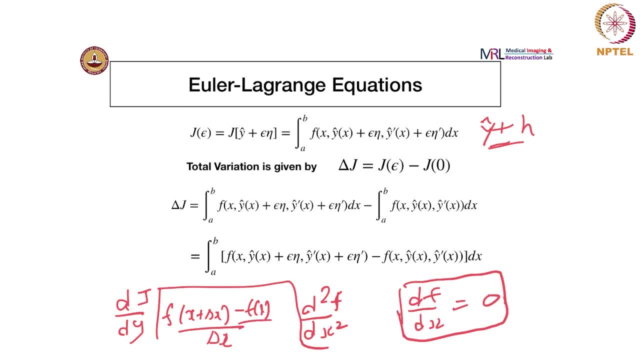 df by dx, right? So that is the idea. So, but then to do that, here, you know, you will do something like this, So you will do something like this, So you will do something like this, So we will re-parameterize so that it is not easier to do. So what you do is, instead of h, 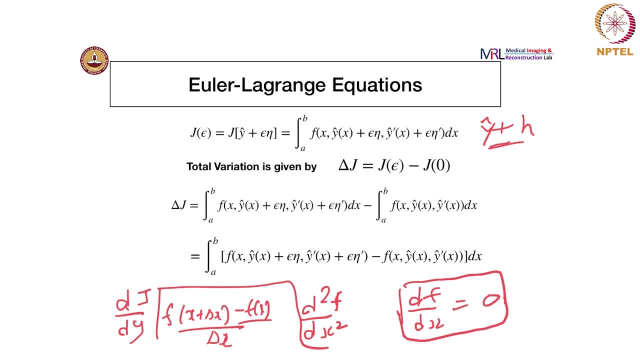 you write y of x plus epsilon eta of x, So that is what we have here this term. So it is epsilon. write it back here: epsilon eta of x, So eta of x can be any function. Of course we assume that. 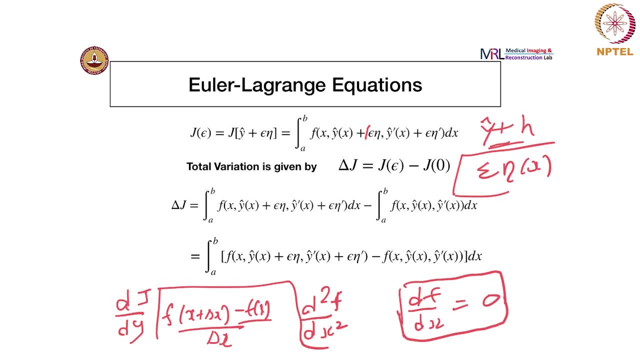 it is typically well behaved that it does not have some nasty discontinuities, but generally, eta is any function, eta of x is any function and epsilon is a very small number. right, The delta is a very small increment that you have to do, So you have to do this, So you have to do this, So you have. 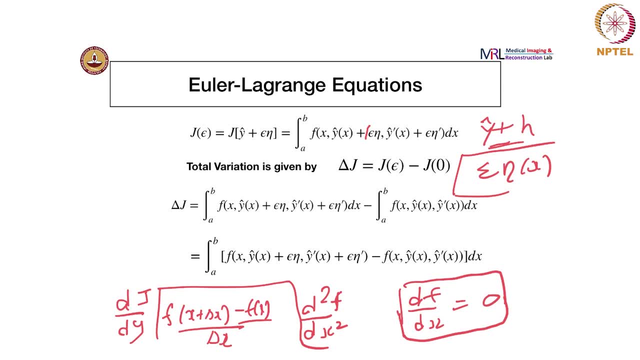 to do this. So this way you can perturb around y hat. right, You can perturb around y hat and see how this changes. So now, j is now strictly a function of epsilon. Why is that? Because y hat is fixed, we now assume that y hat is the correct curve that we are seeking and the curve for which. 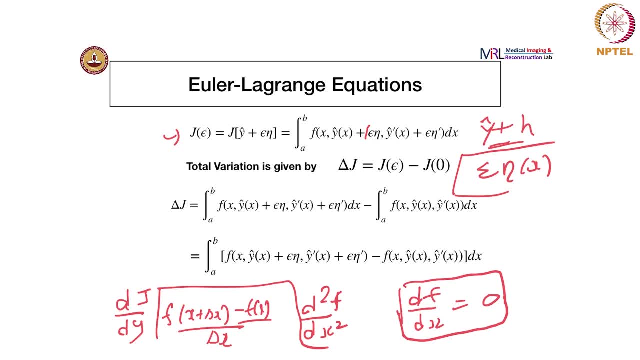 j of y is minimum or j of y, hat is the smallest value j of y can take, and we perturb it with epsilon, eta. We fix eta also. We say it is a test function, It can be any function without loss of generality. we can say It can be any function, eta, and which, of course, 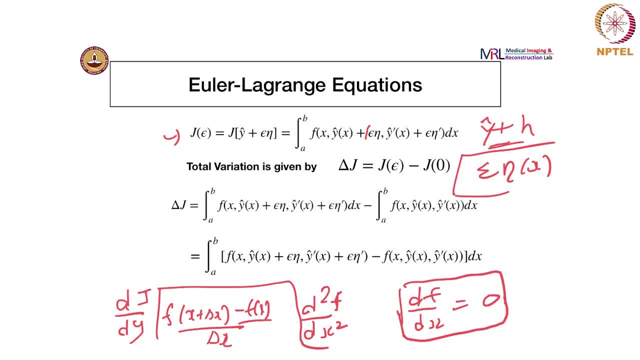 like I said, that is desirable, you know, well-behaved function. We do not want some pathological function right, something that goes into infinity and all that We do not take. We just say, you know, it is a function which is well-behaved because derivatives. 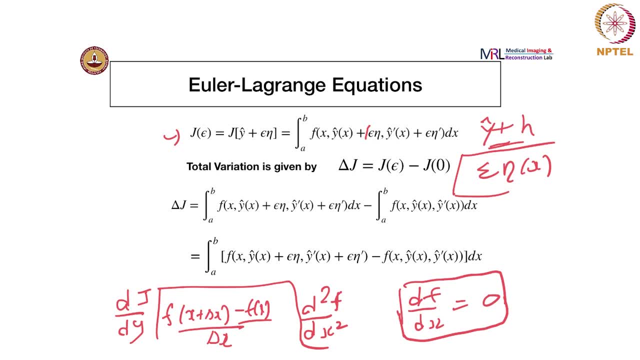 first and second derivatives exist right And then. so then we can just, you know, use that to perturb. So now that is also fixed. So the only thing that we are changing is epsilon. So we are actually searching in the neighborhood of y hat, just making sure that for any such 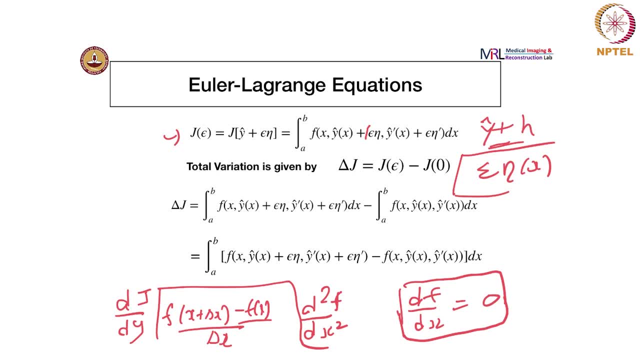 you know value of epsilon. your function takes j. the functional takes higher values than that than at j of y hat. okay, So then we calculate what is known as the first variation And before we do that, define what the total variation is. Total variation is given by this expression: delta. 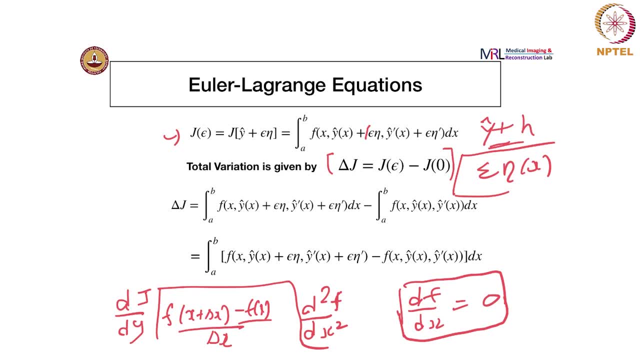 j is j of epsilon minus j of 0. So what is j of 0?? Just put: epsilon equals 0 with just the functional which is estimated at y hat right and y hat of x and y hat prime of x, right. So 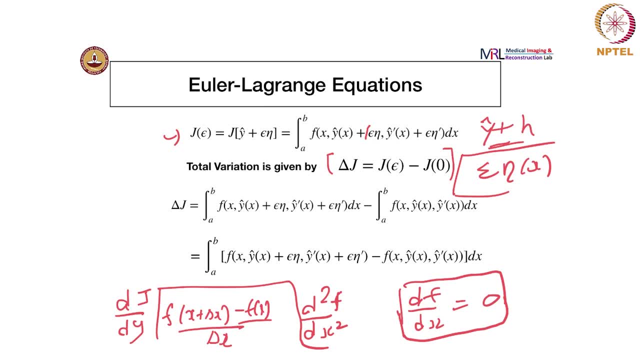 now we can write the total variation in this form: j of epsilon minus j of 0.. I have just substituted for j of epsilon here and j of 0 here. Now the second step is, of course, bring them under the same, make them one integral under the same integral. And if you look at this: 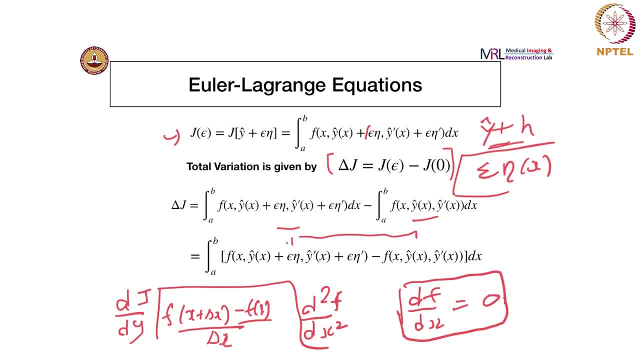 you know you can just then. now you do your usual tricks like you can do a Taylor series: expansion of f of x, y hat of x plus epsilon eta, y hat prime of x plus epsilon eta prime. So you can think of f of x as a. 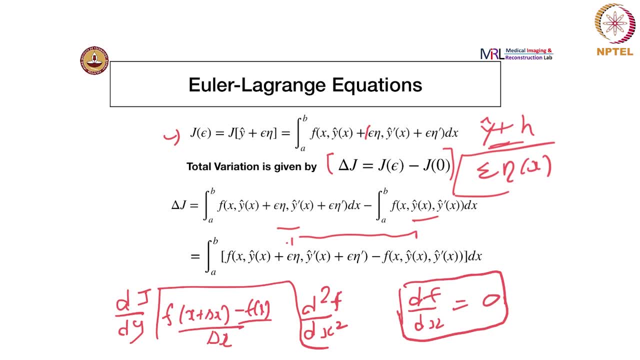 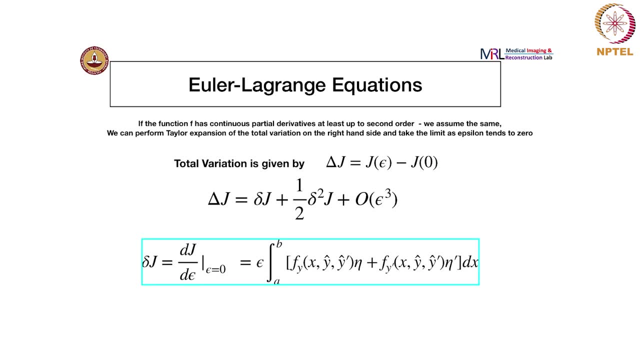 function of several variables and you do a Taylor series expansion. So and then, once you do that, you will see that this term will cancel out and what is remained, which what we will refer to as the. you know you can call it the first variation, The left hand side, also the total variation can. 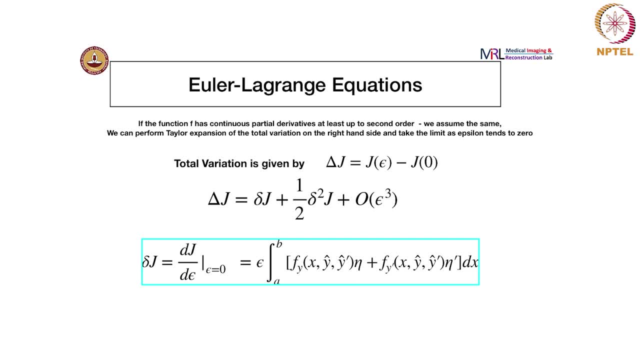 also be expanded into Taylor series And once again, the j of 0 will then subtracted out, because that is what we are expanding around, right around j of 0. And once we do that, then we get this term, which is known as the first. 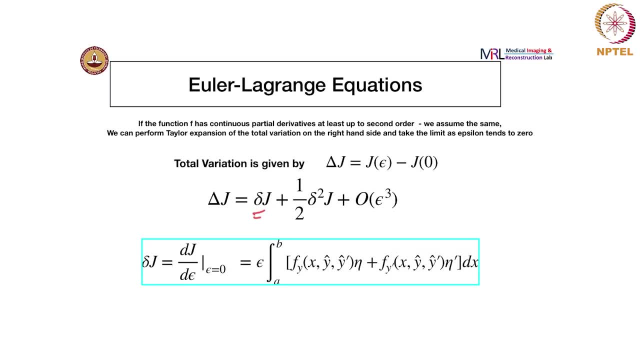 variation. okay, First variation, which is nothing but d, j by d epsilon at evaluated epsilon equal to 0, and it will turn out that it is this expression on the right right And in order for, to order to, for us, for the, for the minimum to occur at y hat. 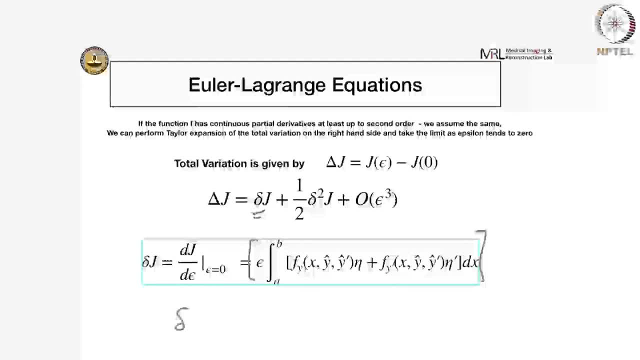 we it should. it turns out that delta j should be 0,. okay, It is not too hard to see because you see the delta, the expression for delta j, is a odd function of epsilon. okay, So if we change the sign of epsilon, okay, then you know you can. then what happens is: 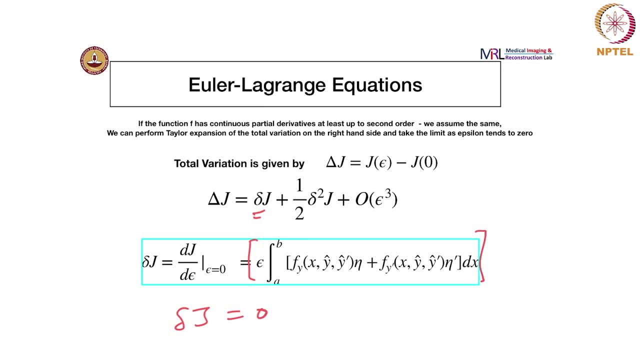 automatically changes the sign here at delta j. See, delta j is j epsilon minus j of 0.. See, this is the minimum right. j of 0 is the minimum, okay, Every. any other perturbation should only increase the value of of j. So but if I change the sign of epsilon, 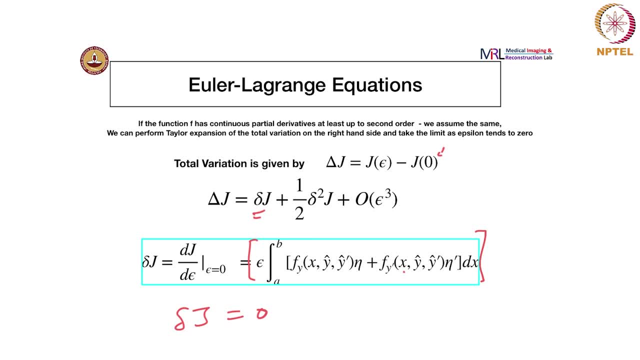 you can show that this will become a positive number. and this say: change the sign of epsilon will change the sign of your, of your, of the value of delta j. So that is, that means that you know you are, you can get higher or lower values. So that is not, that is not correct. 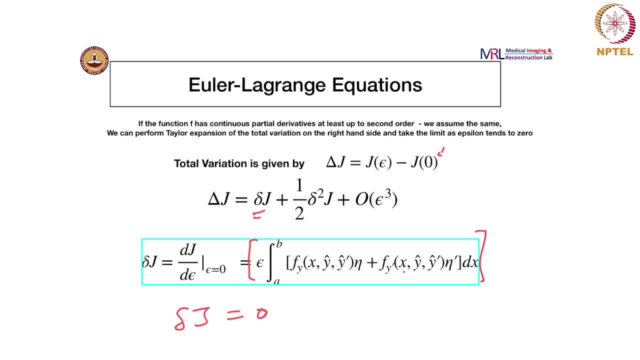 So then you have to set delta j equal to 0. So we can show that delta j equal to 0, that is okay like a theorem you can prove. And once you set that to 0, then the next step. 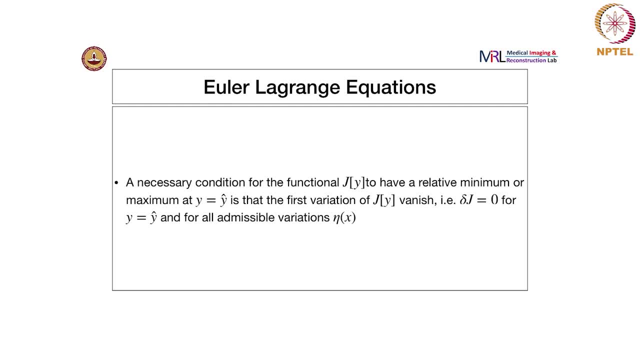 So a necessary condition for the functional j of y to have a relative minimum or maximum at y equal to y hat is that the first variation vanish. okay, So this is like a theorem. I am not going to prove it, but I just gave you like a kind of hand-waving argument, because 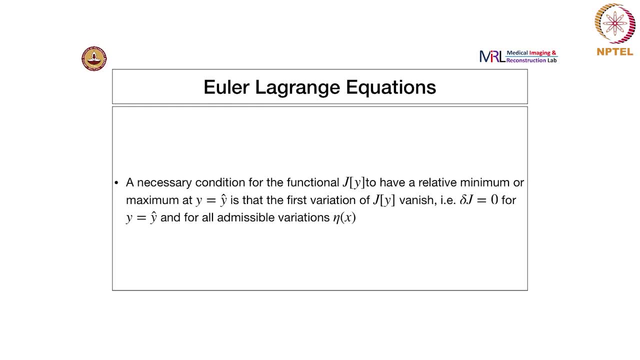 delta j, which is called the first variation, is an odd function of epsilon. okay, So by changing the sign of epsilon we can make it lower than j of 0, which is not true, right? because j of 0. 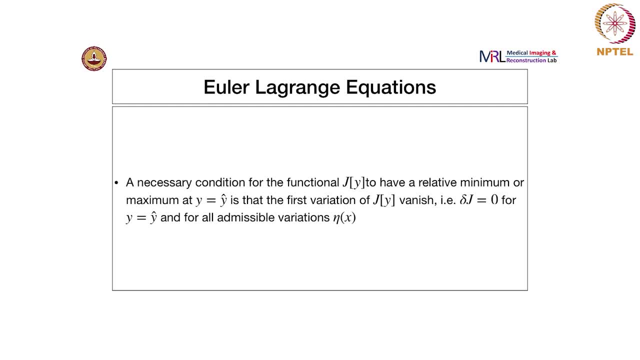 corresponds to y hat, And that is. we know that, I mean we have assumed that way we defined it, is value at the correct or the optimal solution of y. So then by changing the sign of epsilon we can make the total variation positive or negative. So to prevent that, the only way 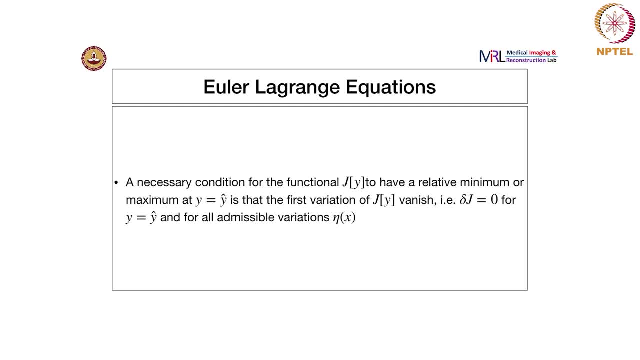 that can be prevented is by making delta j equal to 0,. okay, So the theorem once again is for the necessary condition for the functional to have a relative minimum or maximum at y equal to y hat is that the first variation of j, of y vanish, that is, delta j equal to 0 for y equal to y hat. 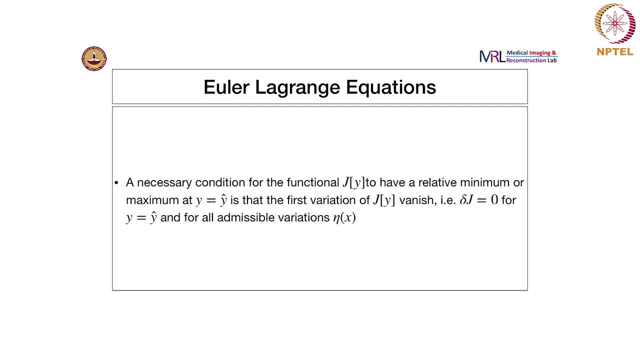 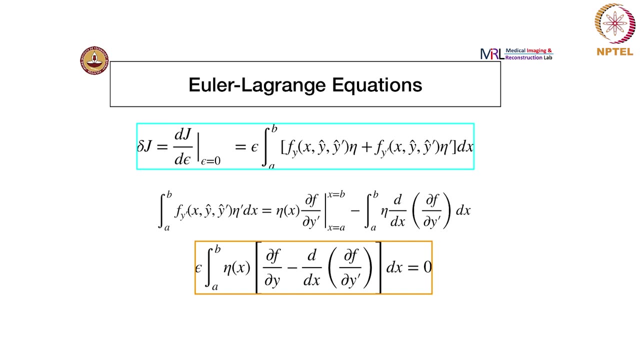 And for all admissible variation, theta of x. okay, So once this is done, then we can go here and look at what happens if we set this to 0, okay, Again, it is another way of looking at it. is that you? 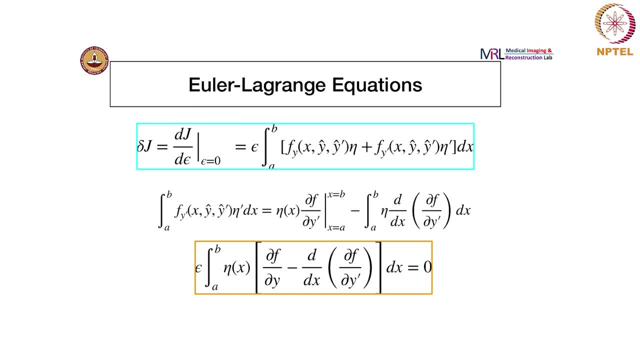 are setting the first derivative to 0. It is an easier way to look at it: Set that to 0, right, And once you set that to 0,. another thing that we have to do is we have to simplify this expression. 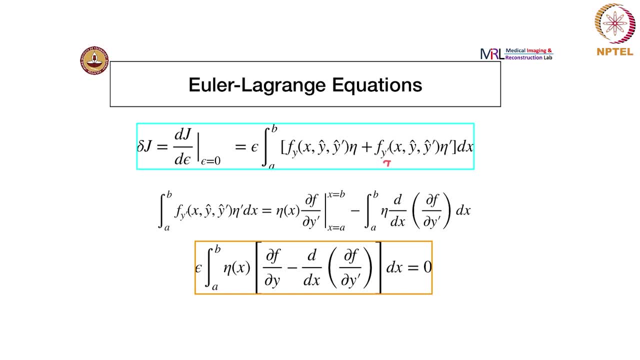 So f of y prime- once again- sorry if I have not mentioned this earlier- f of y, f underscore, sorry, f subscript y is nothing but delta f by delta y, And f subscript y prime is delta f by delta y. So we assume that. So we can do integration by parts. So 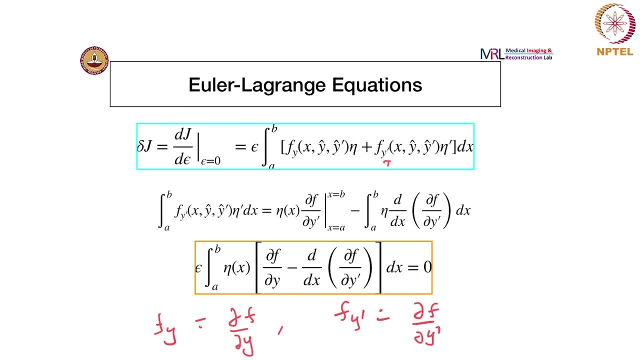 if we take the second expression, we can do integration by parts and use the boundary condition to eventually come at this expression. okay, Now, all you have to do is focus on the term in the brackets. okay, Now it turns out that we can prove, in order for the 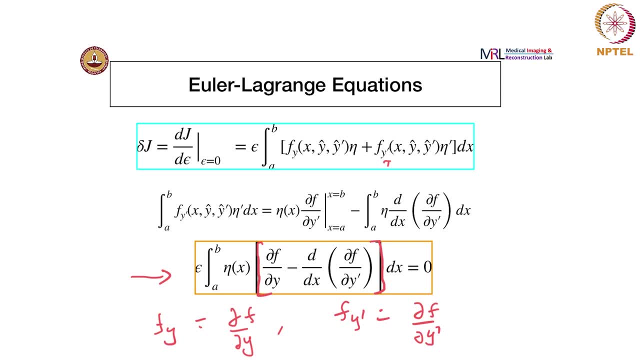 integral to be 0,. right, for any theta x, this term should go to 0.. The term that I have put in red bracket should go to 0,. okay, That is another thing. See that we did integration by part for this f of y prime derivative with respect to y prime. okay, And if you have 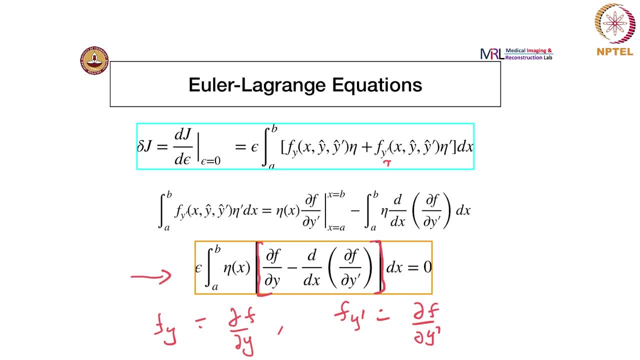 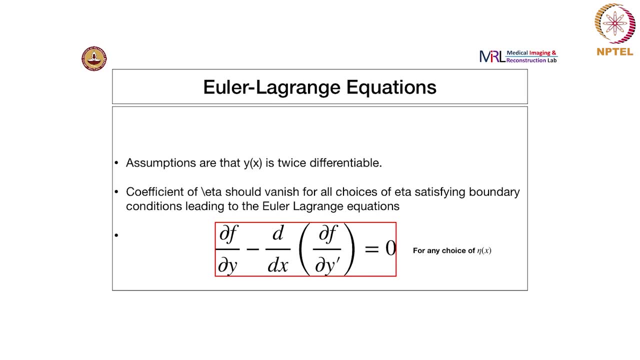 if you have y, we will have a derivative with respect to y w prime. if f is a function of y w prime, then we will have another term. We will have to do integration by parts twice. right, that we can prove. okay. So the coefficient of eta of x. I am sorry there is an error here. 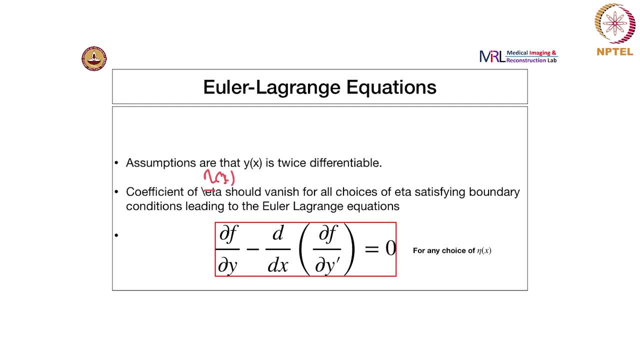 coefficient of eta of x should vanish for, should vanish for all chances of eta satisfying boundary conditions leading to the Euler-Lagrange equation. So these are the Euler-Lagrange equations. So now these equations are partial differential equations. okay, And this is what you use to. 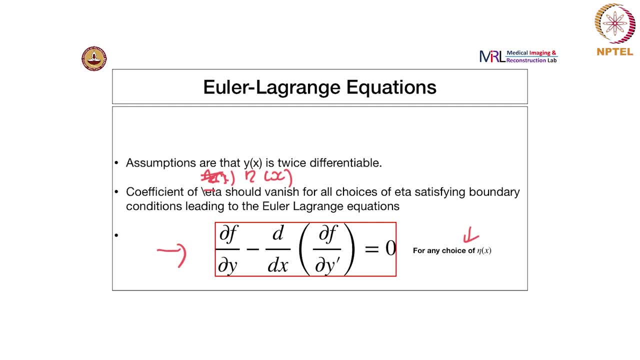 actually estimate y. okay, See, that is a function of both y and y prime And in this case, because we started out with f strictly as a function of x, y and y prime, okay, Sometimes this is also a function of y double prime, which is d square, y by dx square, And in each case there will be an. 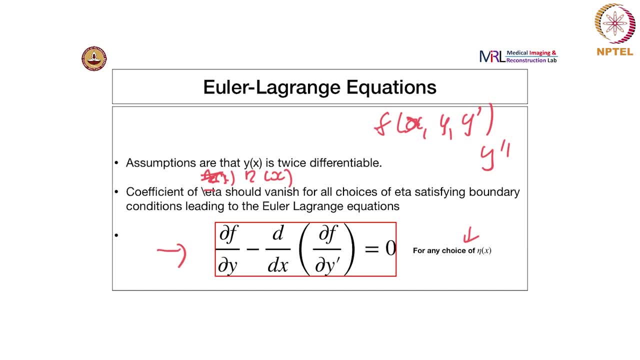 additional term with a change in sign. Okay, so we will look at that in another slide, But that is one of the things that you have to remember. It can also be a function of higher derivatives, And for that so? and what happens? 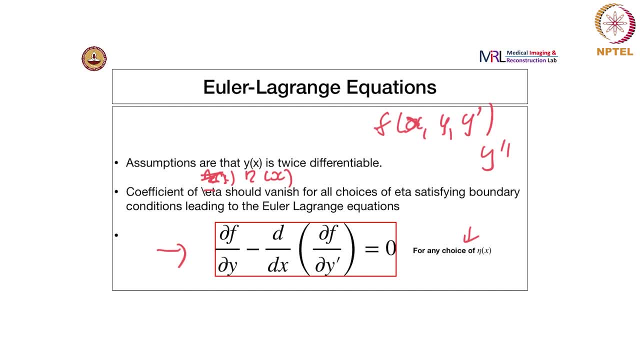 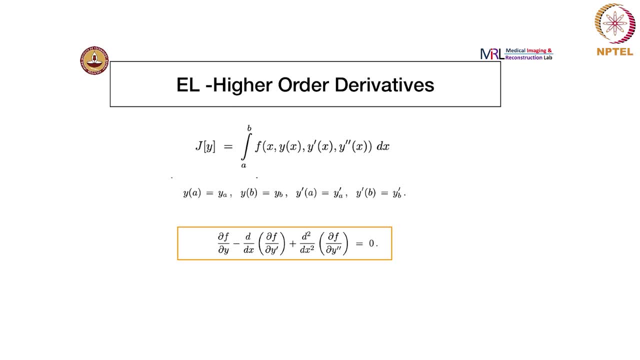 is that, when you want to solve that, if I, if you go back to the previous and so there will be one more term here, we will look at that later. Okay, and that is why here I was talking about if j of. 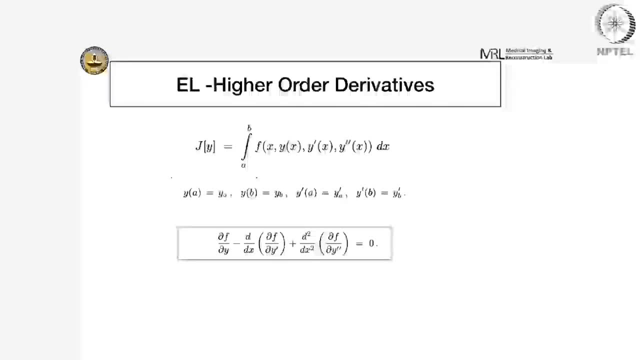 y and where f is a function of y double prime, also here. then you will end up with an equation like this: Of course, the sign will be flipped. note that the sign is flipped Because you will do integration by parts twice and there will be a minus sign, extra minus sign. 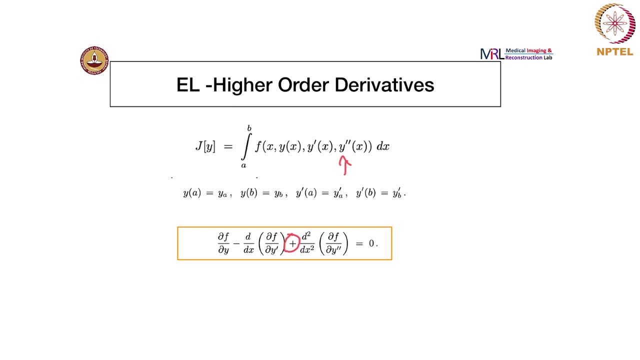 which will make this possible. Okay, so this is the Euler Lagrange equation, And this is what you know is the driver for all the methods that rely on all the PDE based methods and that rely on calculus of variations. So we will look at something called SNAICS- active contours, That is.